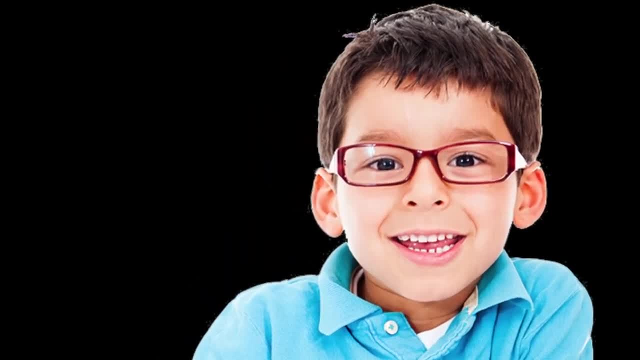 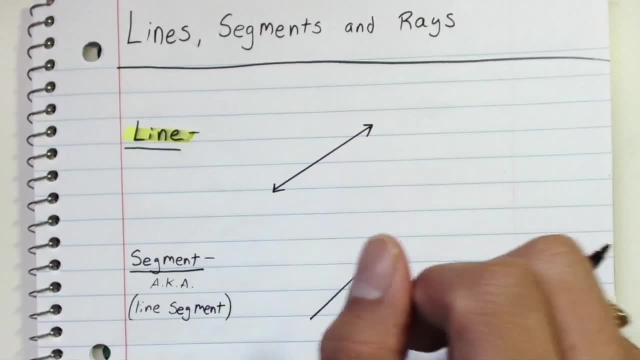 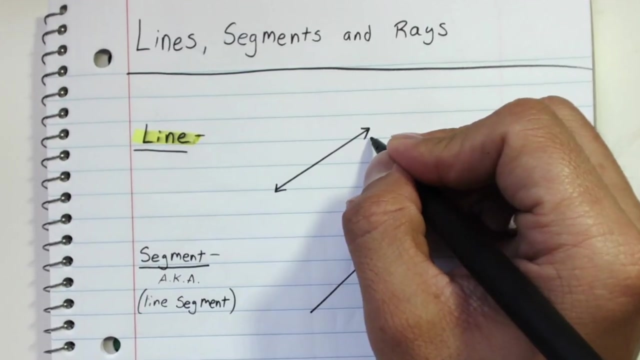 obviously a line, but at the end of it you're going to have little arrows like: so Now, these arrows represent the idea that this line goes forever in both directions. So this arrow is saying that this line goes forever and ever and ever past this paper, past my room. 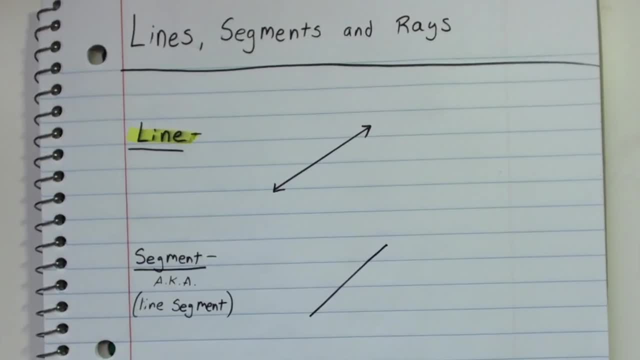 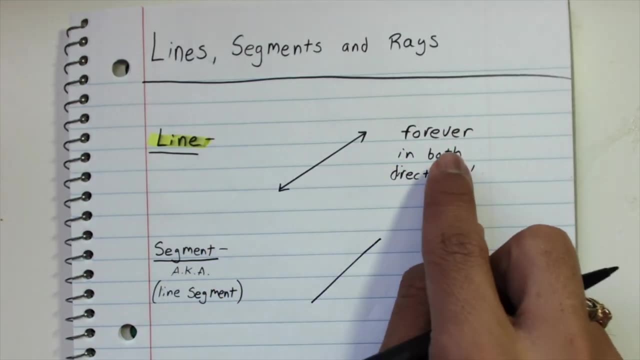 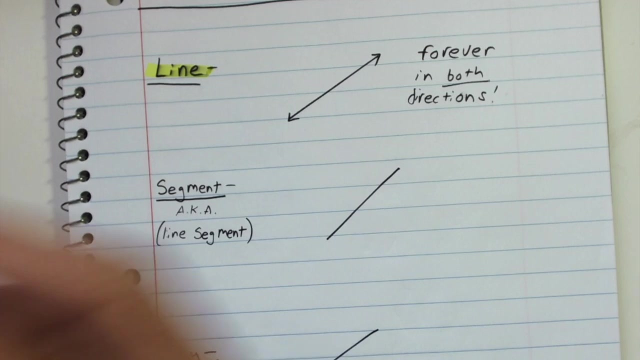 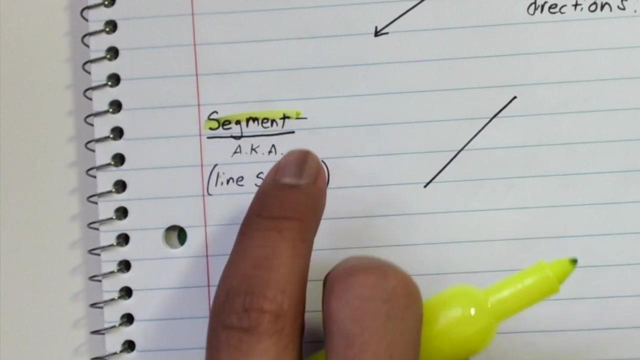 past, you know, the next city, over into infinity. It just goes on forever and ever. A line goes forever in both directions. Keyword both. Now moving on to a segment also known as a line segment. With that word you can kind of get the idea that segment means a piece, a part. So 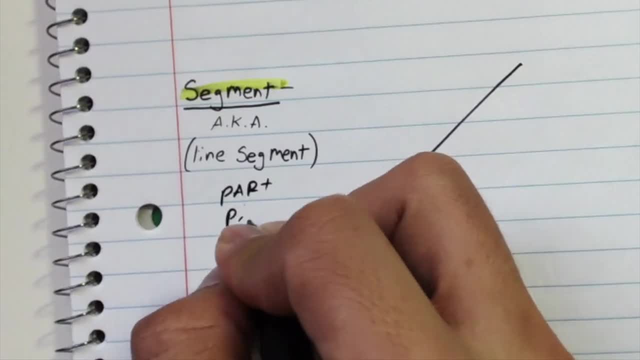 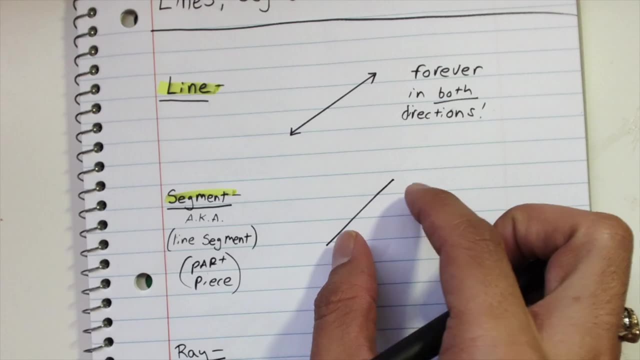 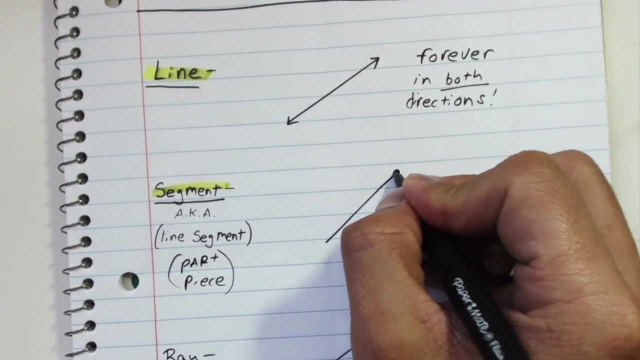 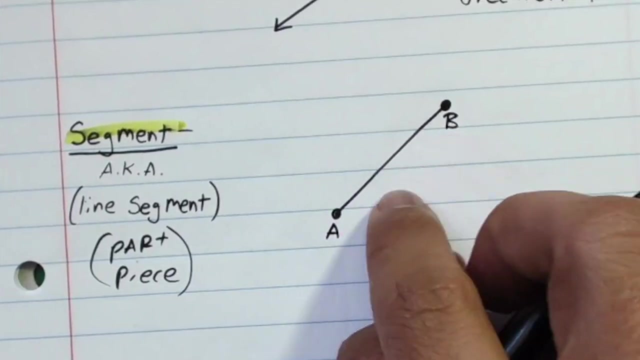 segment would mean part or piece. So if it's a part and piece of a line, then this line segment is. as if I was to take a piece of this line, it would be this Now to represent that we have these two points right here. Let's say this is A and this is B. These two points are where the line 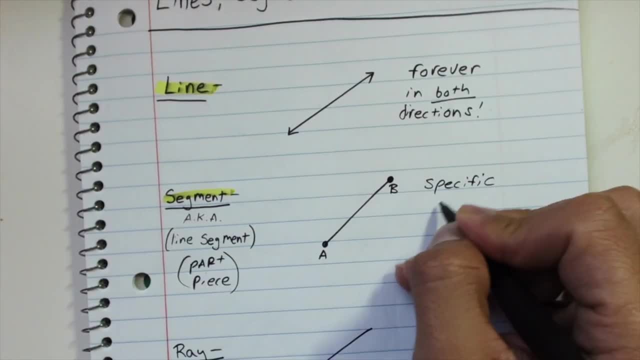 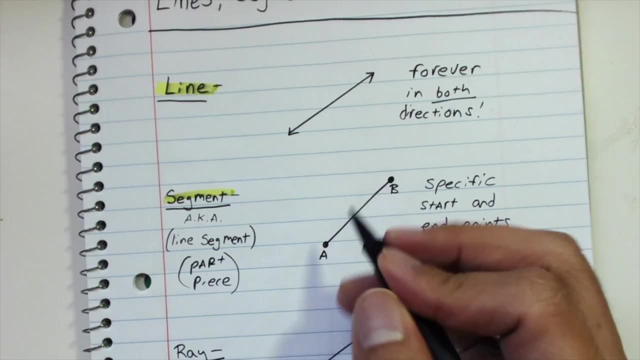 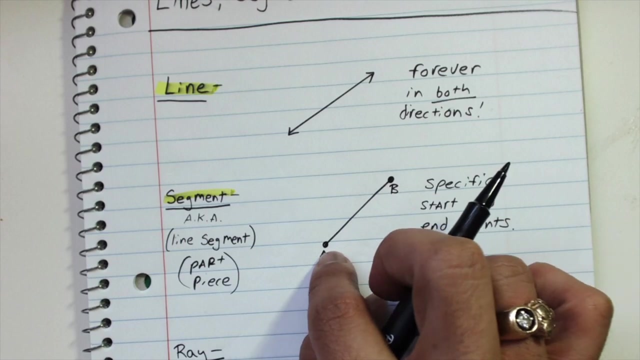 ends. So it has so specific start and end points. The line goes and stops right here. So, unlike a line, those go forever in both directions. This one stops here at B and this one stops here at A, So it's also like a piece of this line, a segment, a portion. 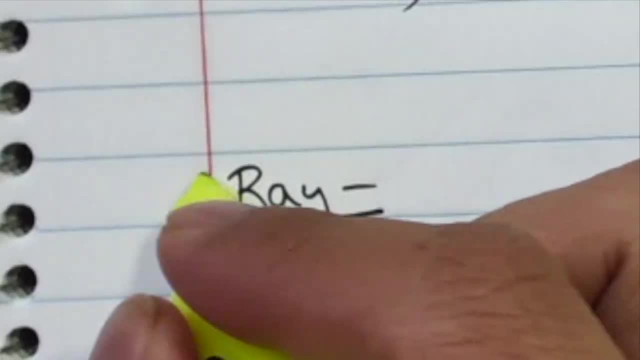 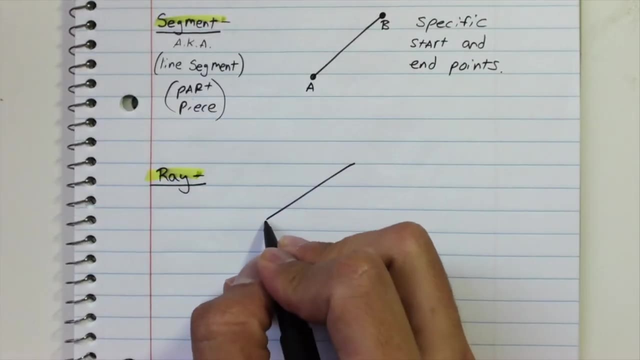 Now, moving on to the final one, we have ray. Now, this idea is kind of similar to both of these. If you were to take both of these, you have a point right here. Let's call it C, And then the other part of the line. 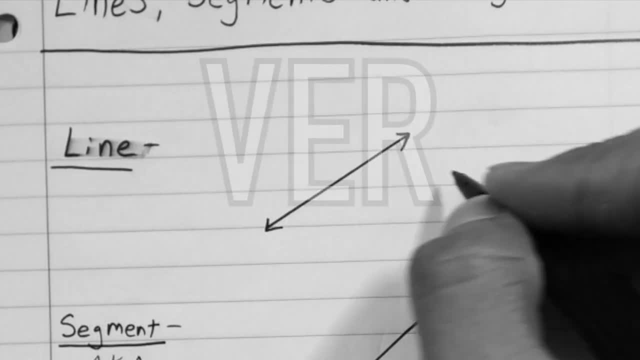 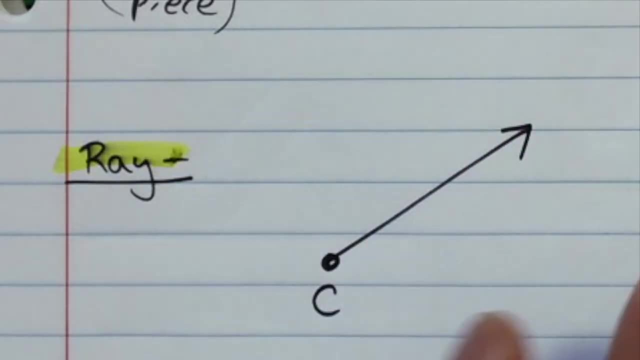 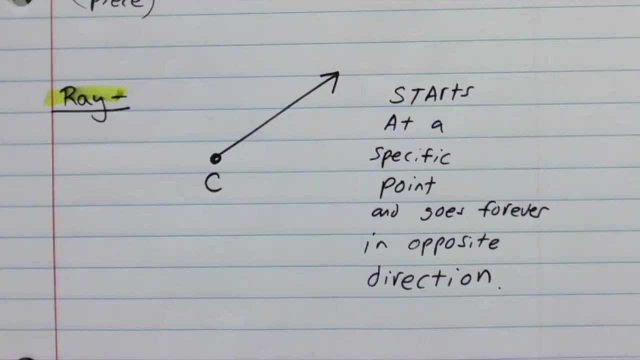 goes forever in one direction. So you see, you have the line going in both directions. This one stops at a certain point and this one's a combination of both. You have it starts here and it goes forever in that direction. That's what a ray is. It starts here and then it goes in this direction forever and ever. 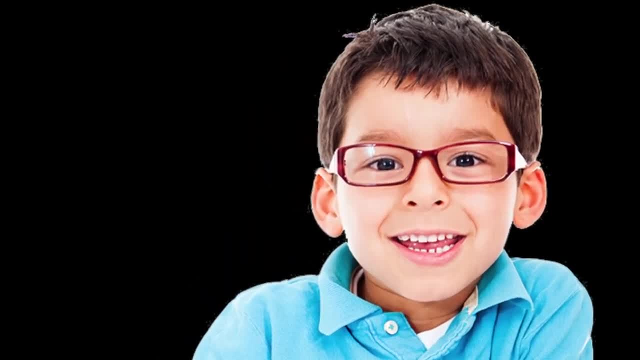 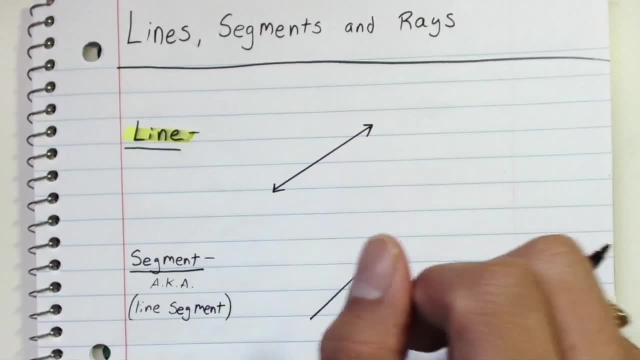 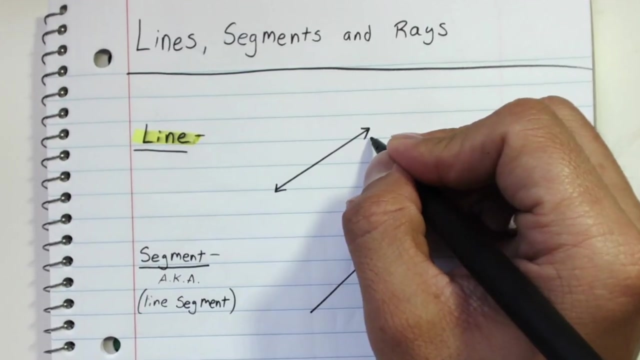 obviously a line, but at the end of it you're going to have little arrows like: so Now, these arrows represent the idea that this line goes forever in both directions. So this arrow is saying that this line goes forever and ever and ever past this paper, past my room. 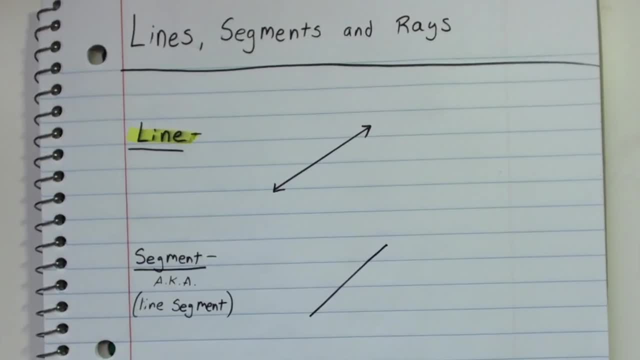 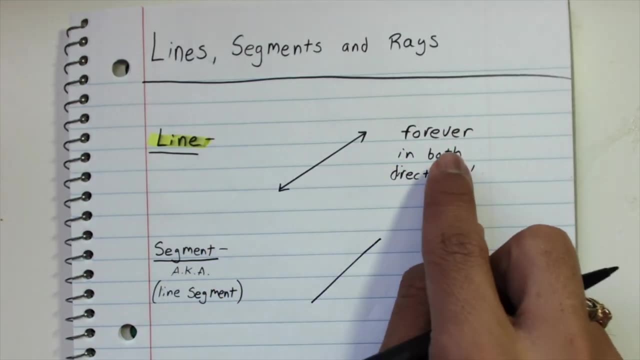 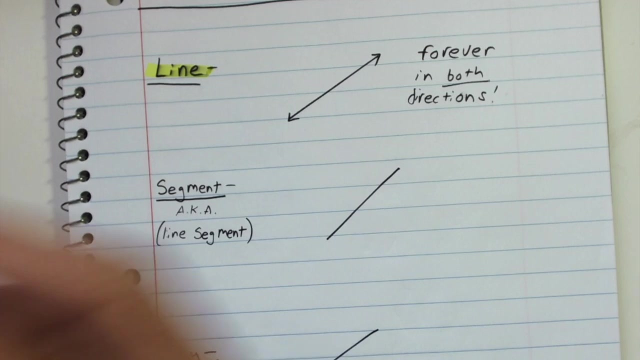 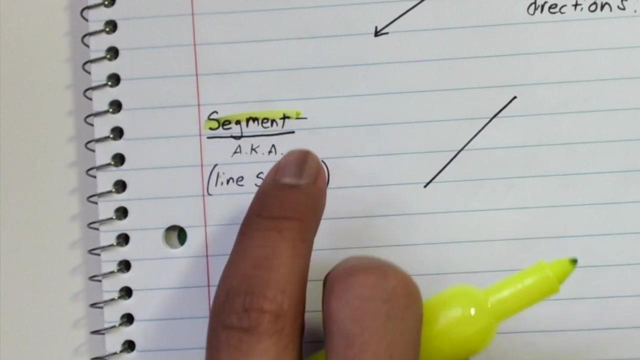 past, you know, the next city, over into infinity. It just goes on forever and ever. A line goes forever in both directions. Keyword both. Now moving on to a segment also known as a line segment. With that word you can kind of get the idea that segment means a piece, a part. So 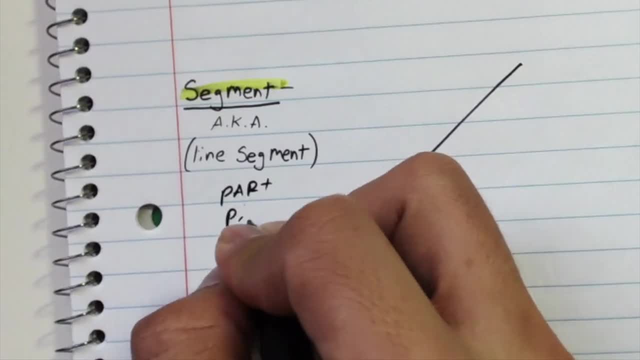 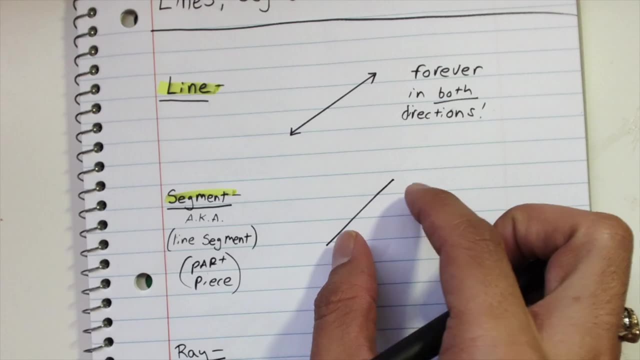 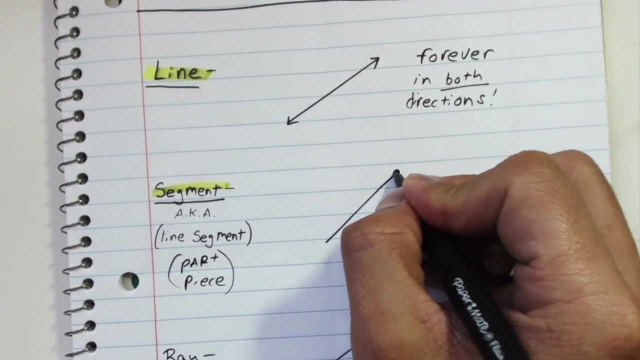 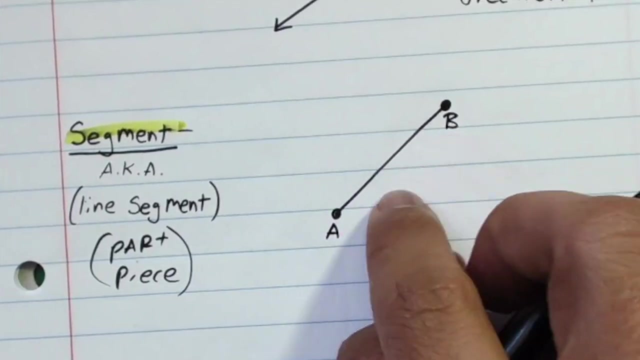 segment would mean part or piece. So if it's a part and piece of a line, then this line segment is. as if I was to take a piece of this line, it would be this Now to represent that we have these two points right here. Let's say this is A and this is B. These two points are where the line 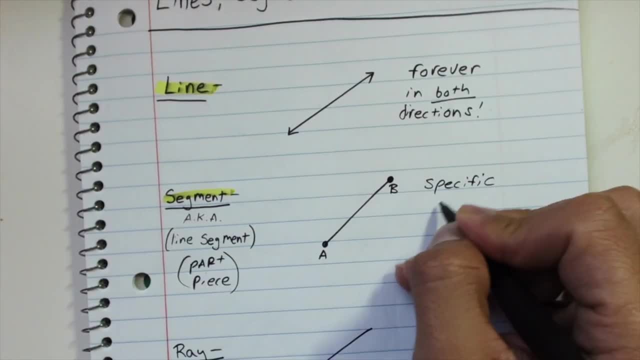 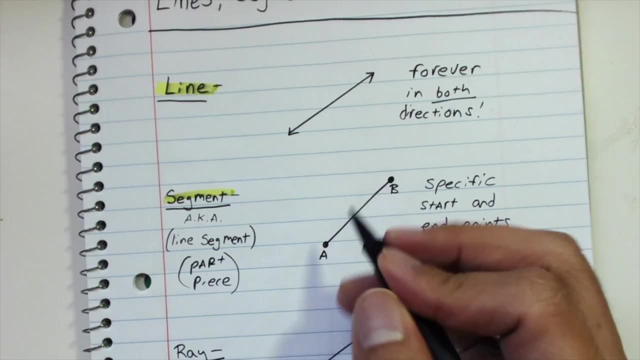 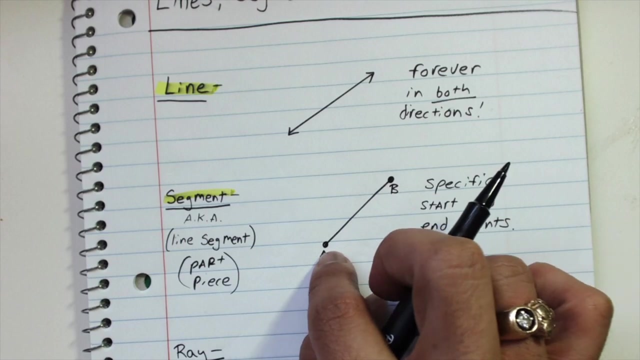 ends. So it has so specific start and end points. The line goes and stops right here. So, unlike a line, those go forever in both directions. This one stops here at B and this one stops here at A, So it's also like a piece of this line, a segment, a portion. 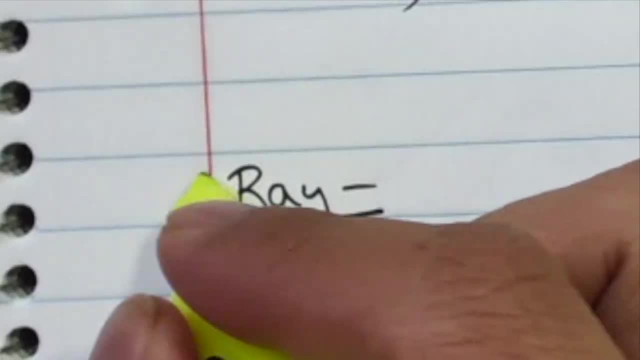 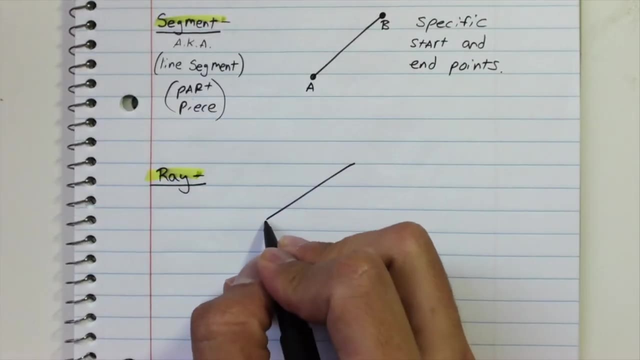 Now, moving on to the final one, we have ray. Now, this idea is kind of similar to both of these. If you were to take both of these, you have a point right here. Let's call it C, And then the other part of the line. 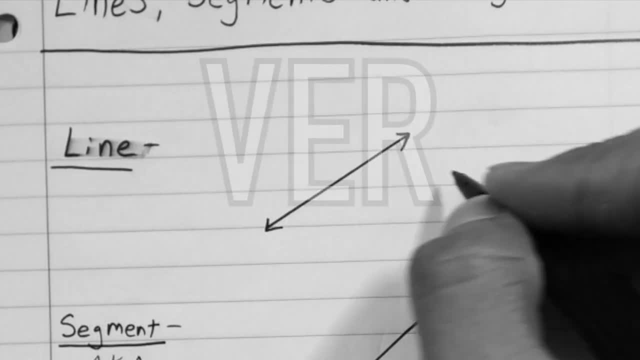 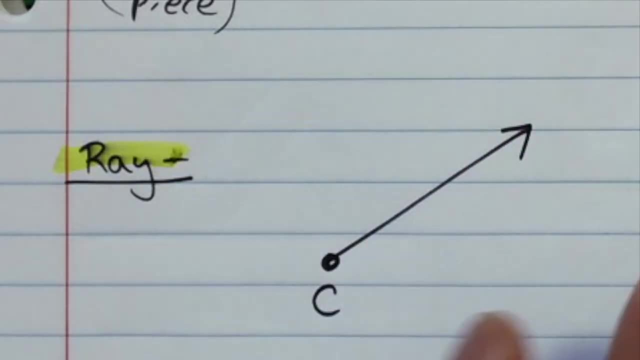 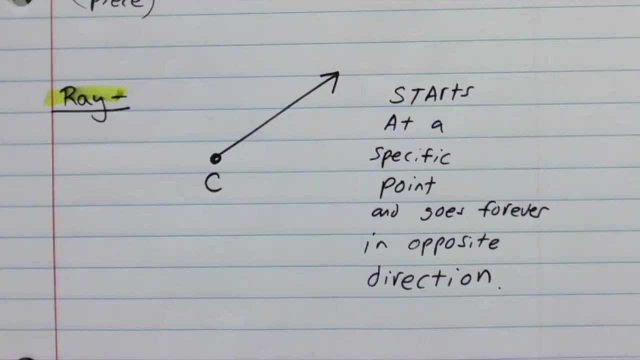 goes forever in one direction. So you see, you have the line going in both directions. This one stops at a certain point and this one's a combination of both. You have it starts here and it goes forever in that direction. That's what a ray is. It starts here and then it goes in this direction forever and ever.